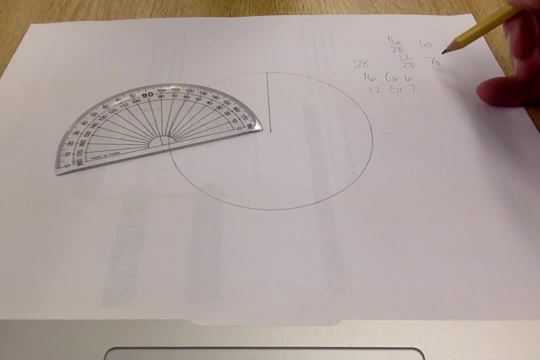 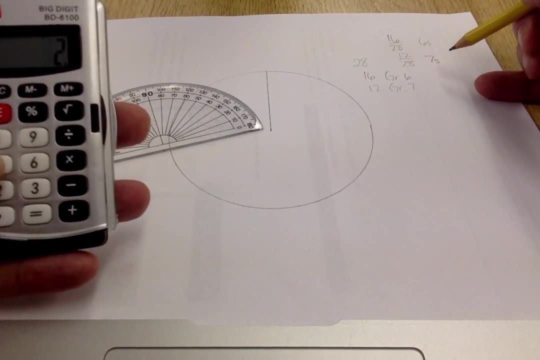 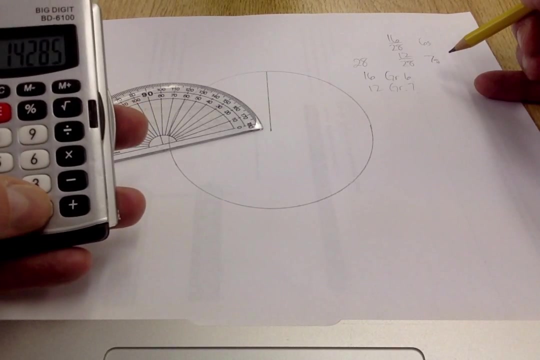 I need to find the percentages of these. so I take my calculator and I do: 16 out of 28 are 7s. I'm going to do: 16 divided by 28 equals 57 and I'm going to multiply that by 100 to give me roughly 57%. 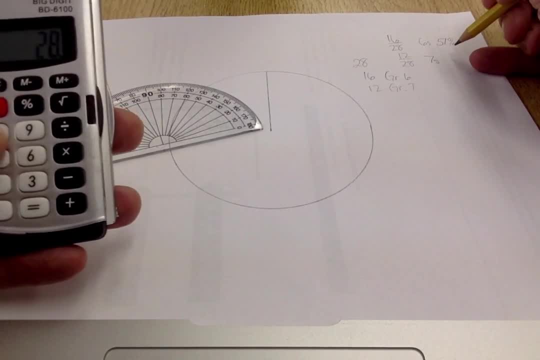 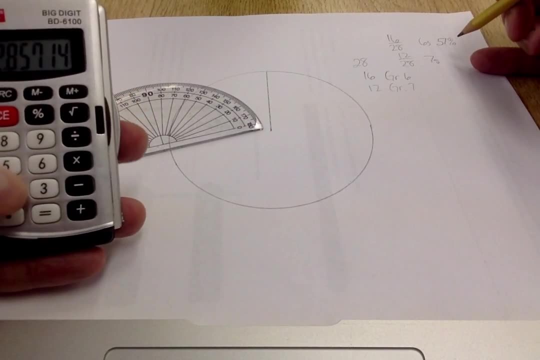 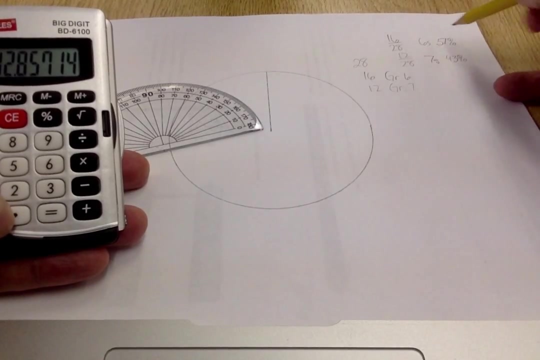 I'll do: 12 divided by 28 equals 42.8 times 100 equals. I'm going to round this off from 42.8 to 43.8.. So there are my percents for the grade 6s and the grade 7s. 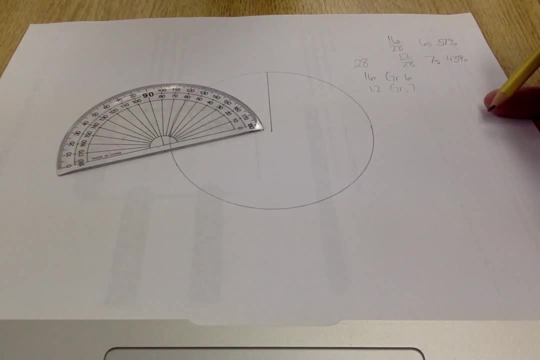 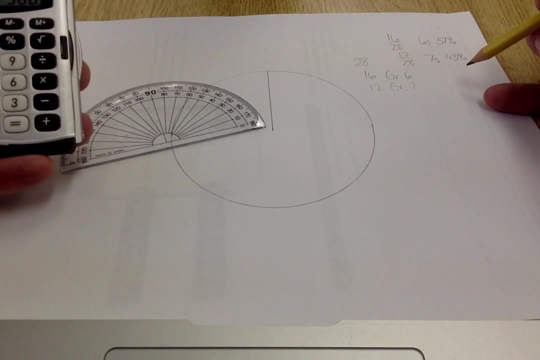 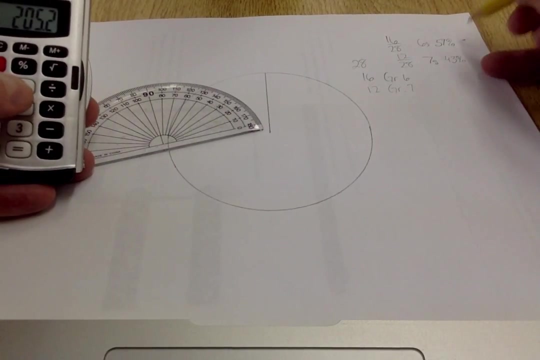 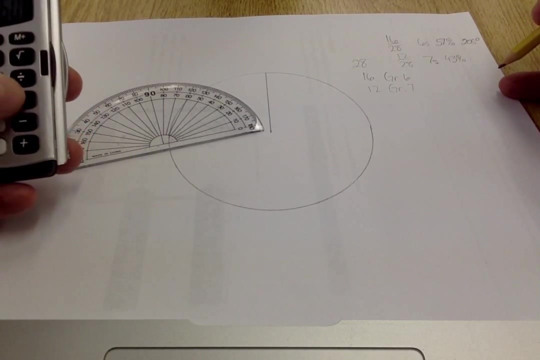 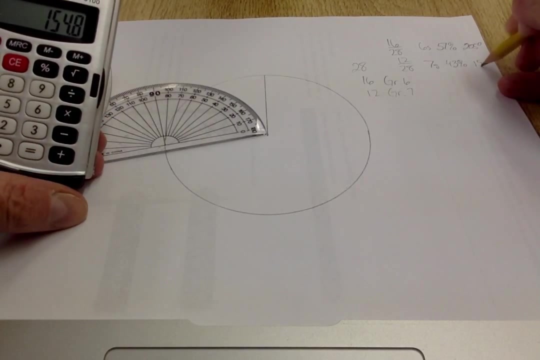 I then need to take my information and convert it so I can use the degrees on my protractor. So I'm going to do 360 times 57%, which is 205 degrees And 360.. Another way to do this is just times 0.43 equals 155. 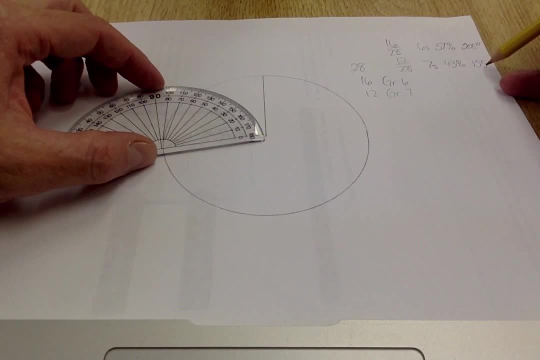 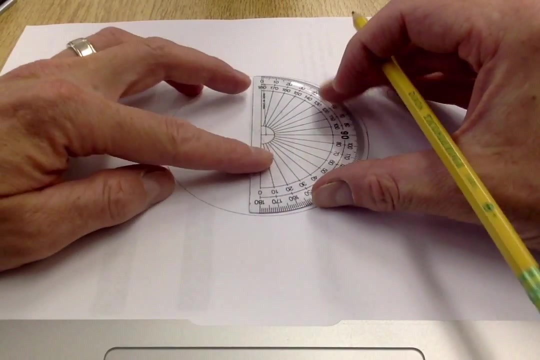 Armed with this information, I have two angles that I need to make, So either a 205 degree or a 155 degree. I'm going to make a 155 degree angle first, So I'm going to put my protractor so that the line that I have already drawn 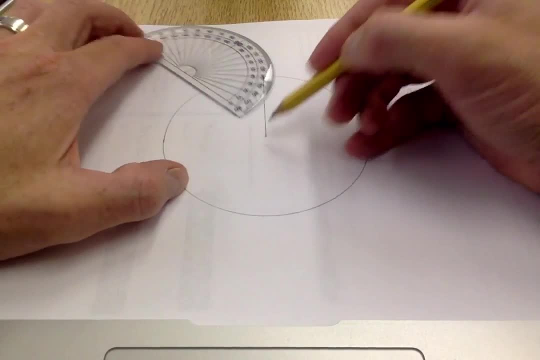 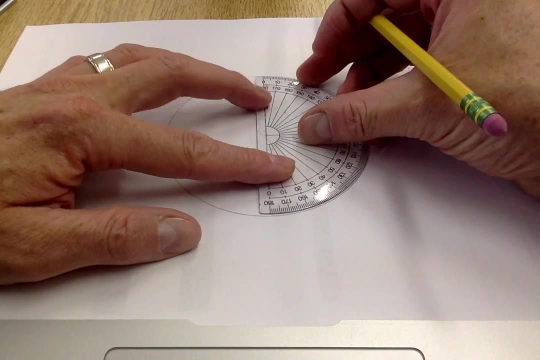 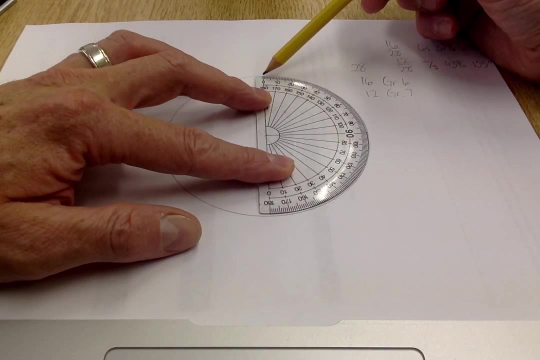 ends right where the protractor has the upright line from 90 meeting the bottom line, Just like that. My first one that I'm going to do. my first measurement is 155 degrees. I'm going to start at the 0, which, in this case, is on the outside. 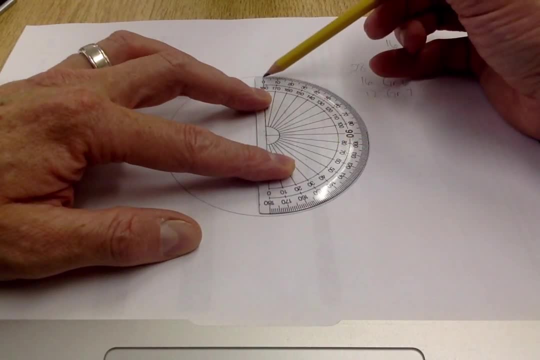 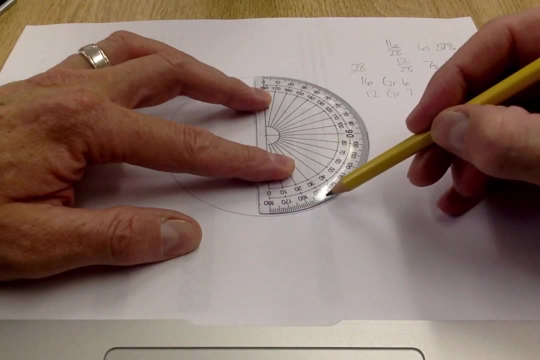 as opposed to the 0 which is on the inside. I need to start at 0 and I'm going to count up 10, 20,, 30,, 40. All the way up to 155 degrees. I put a little dot there. 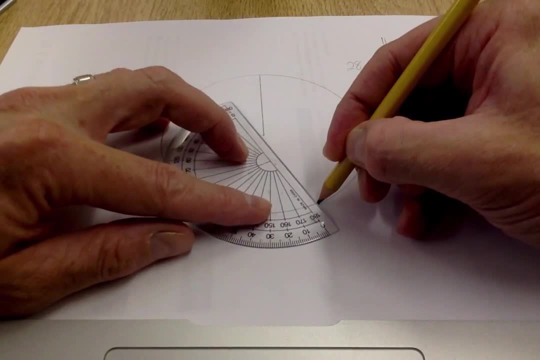 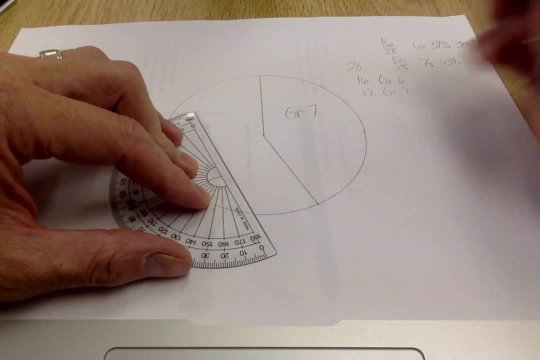 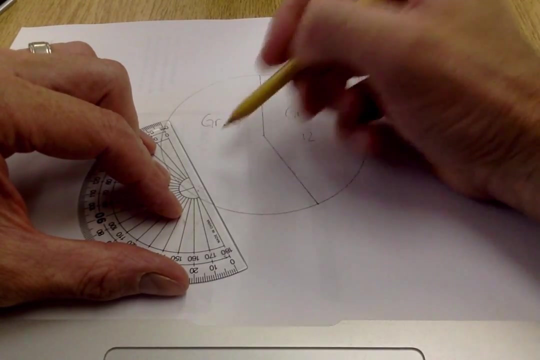 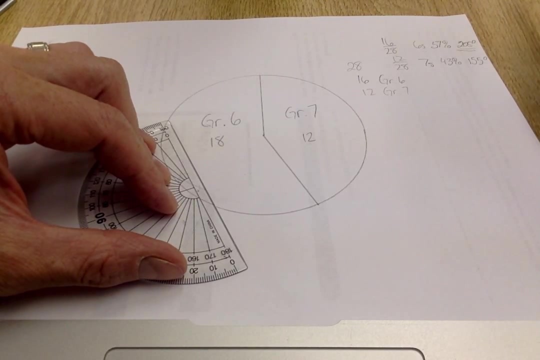 And I connect those dots. So this section here is grade 7.. I have 12,, which leaves me with this Grade 6,, which is 18.. Now let's say you had instead decided to do your 205 degree angle first. 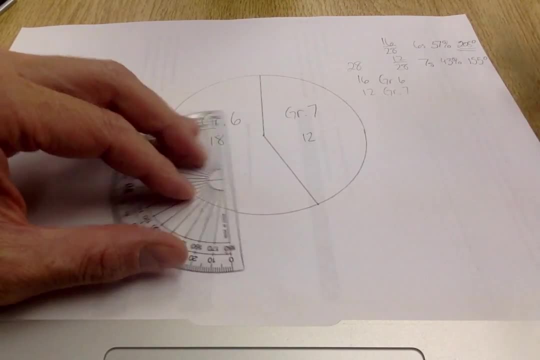 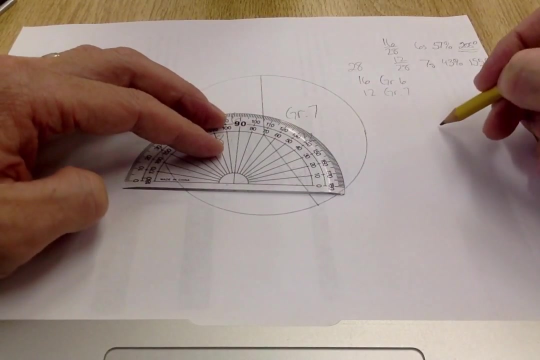 Some of you have said: how is it that I'm going to do it if it's going to be more than 180 degrees, Because my protractor stops at 180!. You have two ways of doing that. You can either do 360 minus 205,. 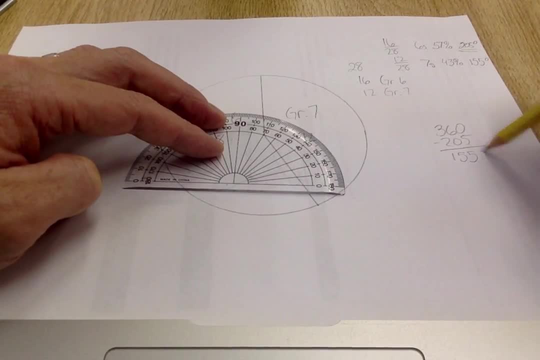 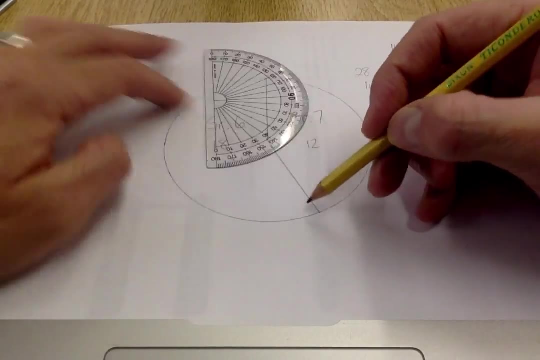 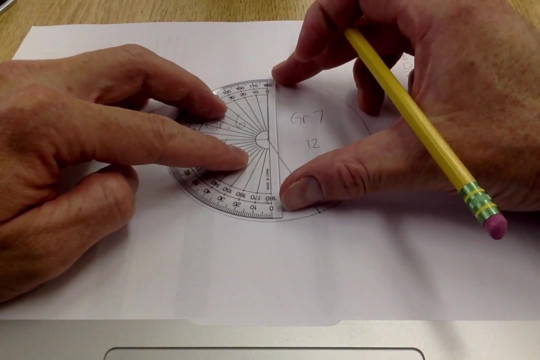 which is going to give you 155. And you're going to measure this angle out instead, which is what we did over here: Measuring out our 155, recognizing that the rest is what's left, Or you can take your protractor. 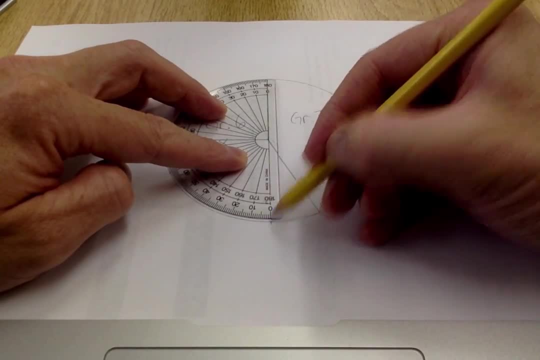 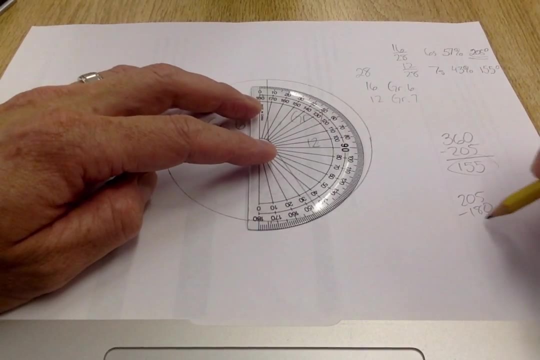 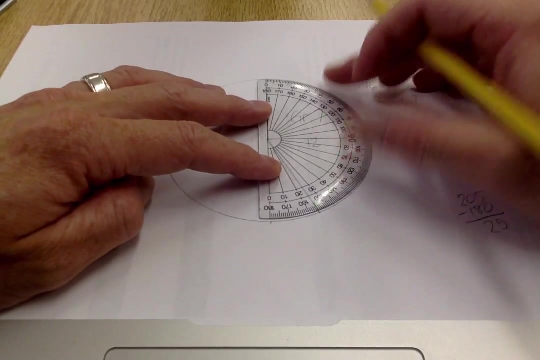 measure out 180 degrees, which would be right here, Because 205 minus 180 is 25.. So I need to add another 25 degrees to this. So I'm going to start over here: 10,, 20,, 5..